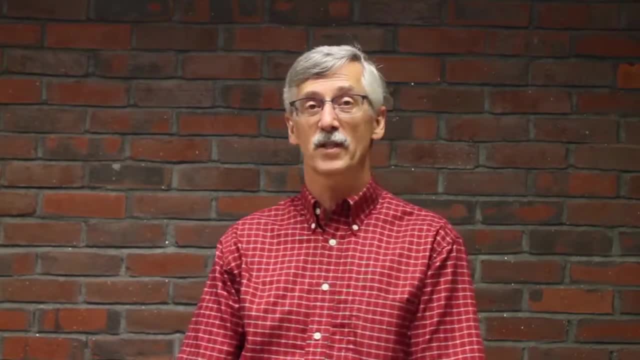 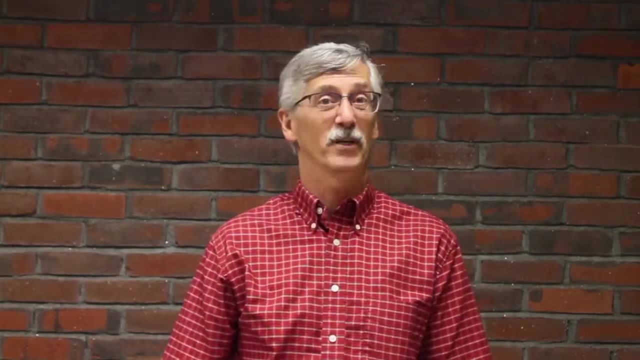 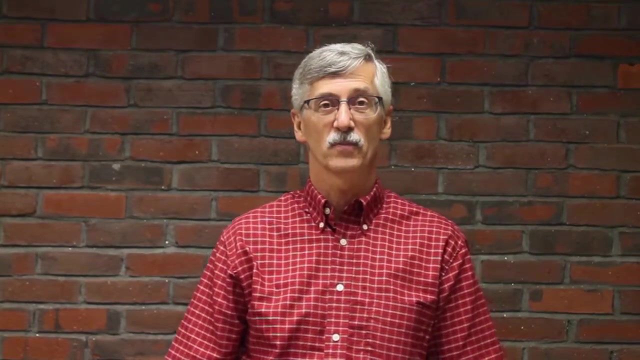 And we say: something is a regulated ignitable waste if it catches fire very easily. But the big question is: how easily do we mean when we say very easily? Well, we have a lab test that actually tells us how ignitable something is. It's called the flash point. 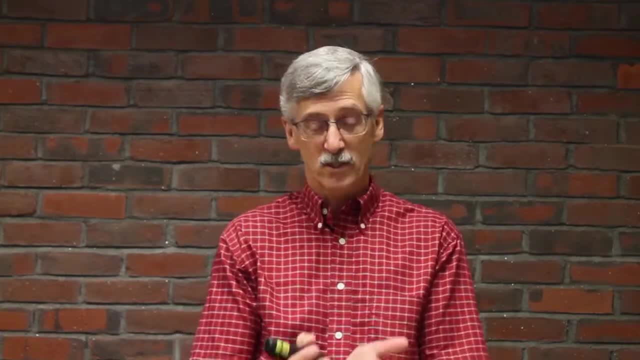 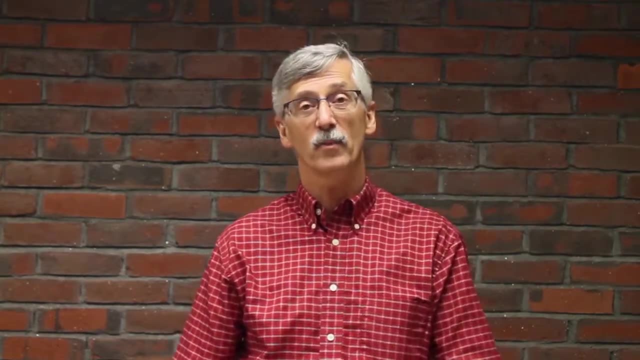 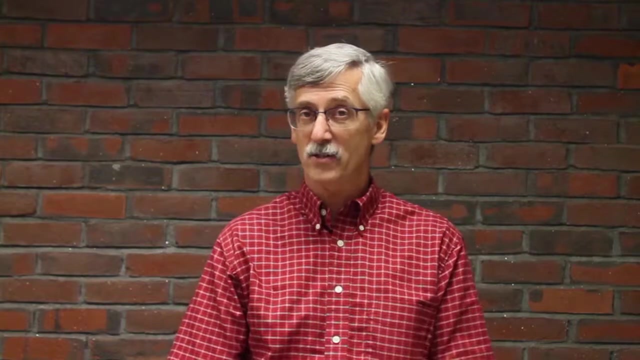 test. Basically, they take a liquid waste and they put it in a metal cup and they heat it up so that more vapors will come off of it. The more you heat it up, the more vapors will evaporate from the liquid. While they're heating up the liquid, they're trying to set it on. 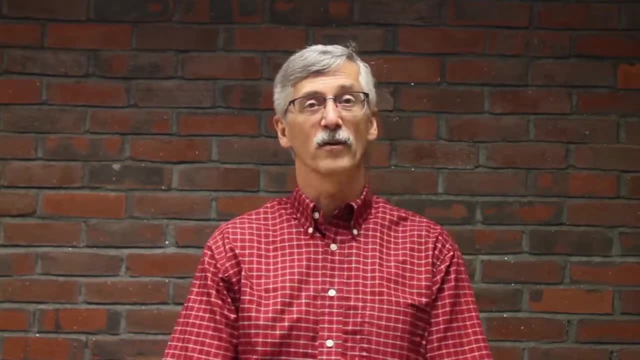 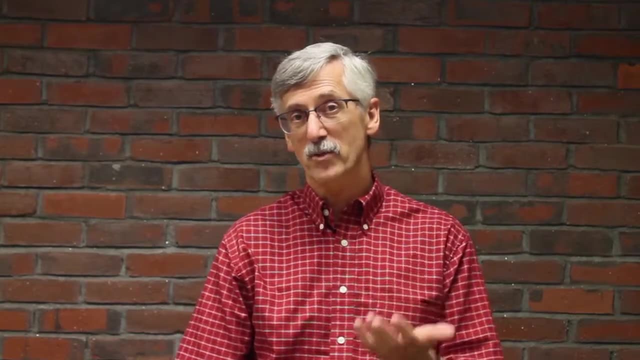 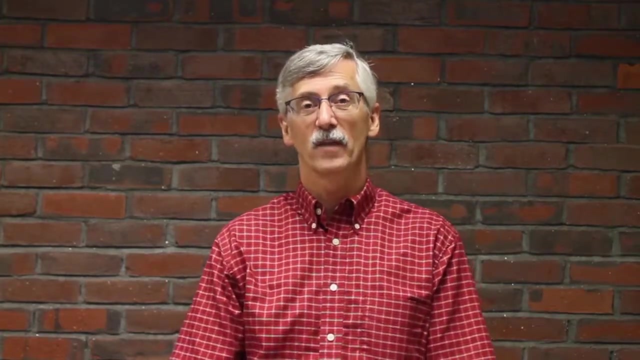 fire with a small flame or barbecue igniter like device. Subtitles by the Amaraorg community. If at some point they heat it up enough that there are enough vapors coming off the liquid that when they try to set it on fire it does, it flashes the vapors they say they've reached. 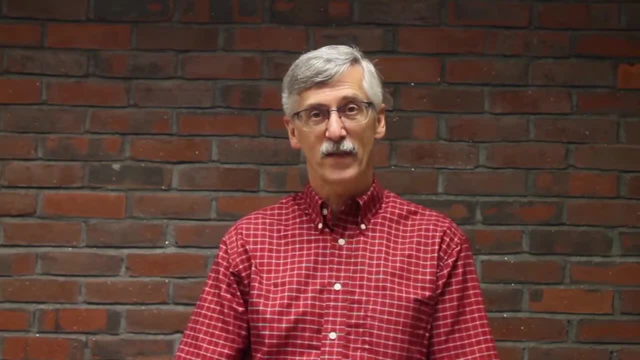 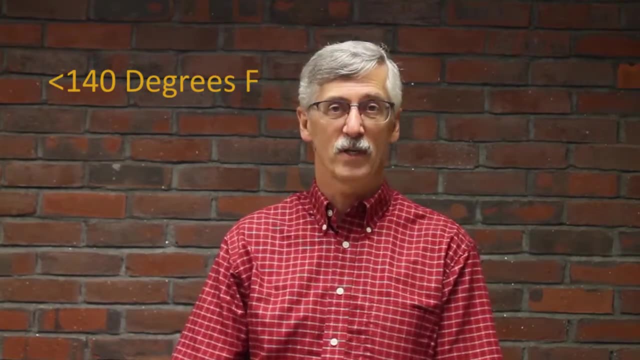 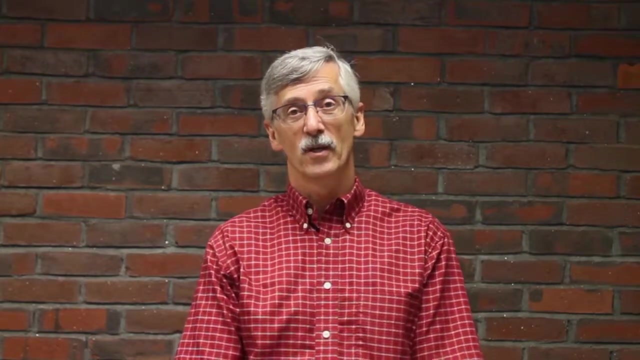 the flash point. They look at the temperature of that liquid and if it is less than 140 degrees Fahrenheit, then we consider it to be an ignitable, hazardous waste. Now it's also possible for solids to be hazardous for ignitability. We say essentially that if something, if it's 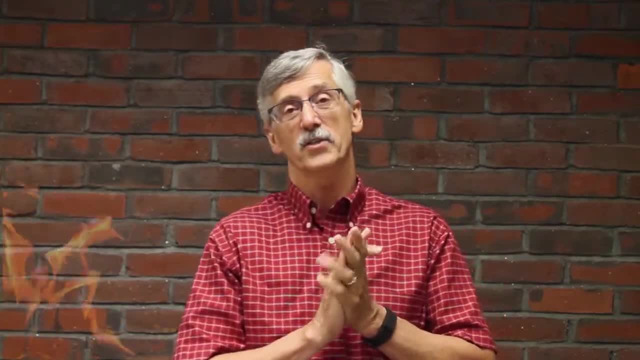 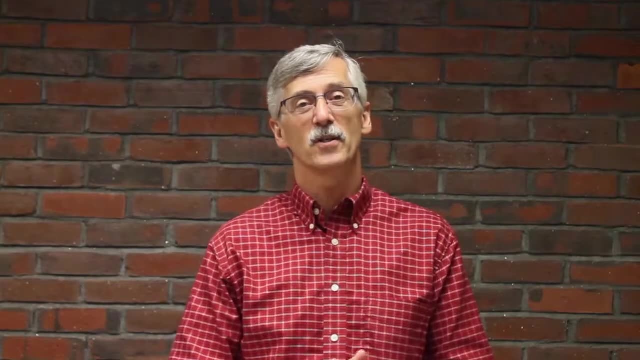 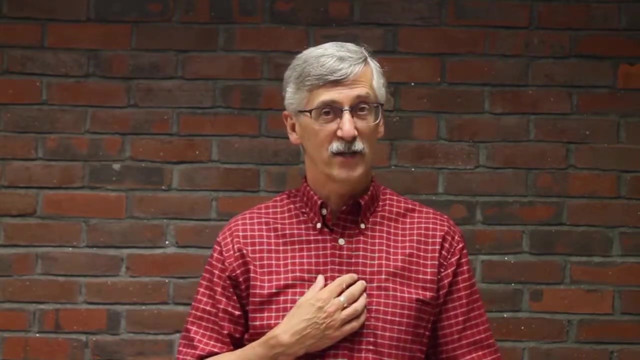 able to catch fire by friction and then, once it catches fire, it really takes off. it's considered to be an ignitable solid waste. If USDOT refers to a waste as a flammable gas, then we would say that is an ignitable waste. If USDOT considers a waste to be an 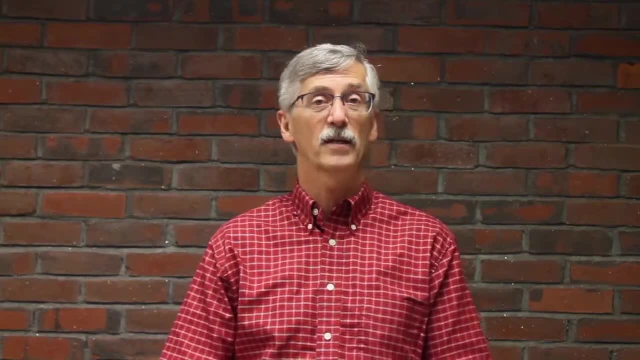 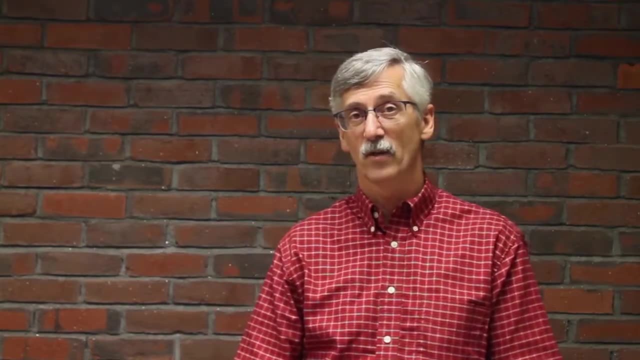 oxidizer. we again would call it an ignitable, hazardous waste. Remember it has to be a waste, not a product. If you're still going to use it, we would not regulate it. Here's a couple of symbols to help you identify in your 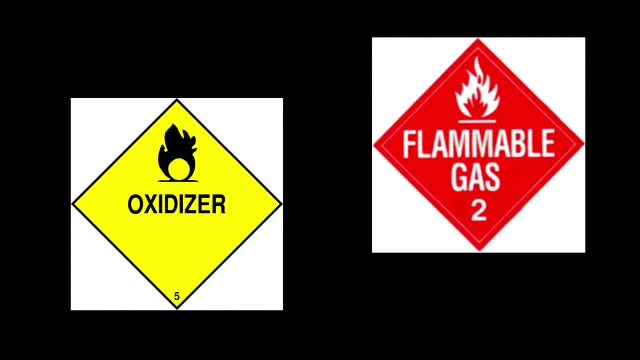 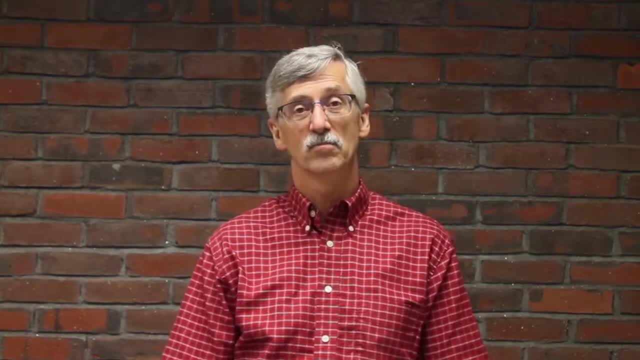 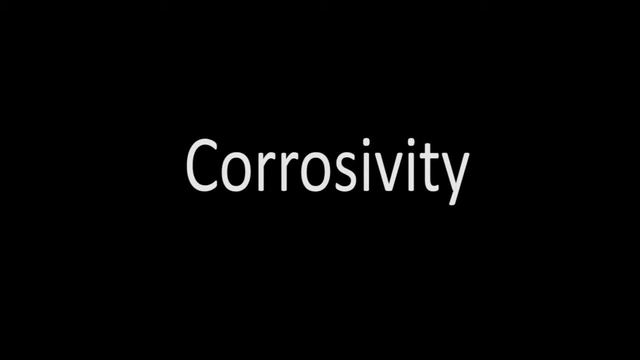 building if you have materials that may be oxidizers or flammable gases. If you see these symbols, just ask questions: Is it a waste? If so, we may regulate it. Our second characteristic is corrosivity- something with a very high pH that we 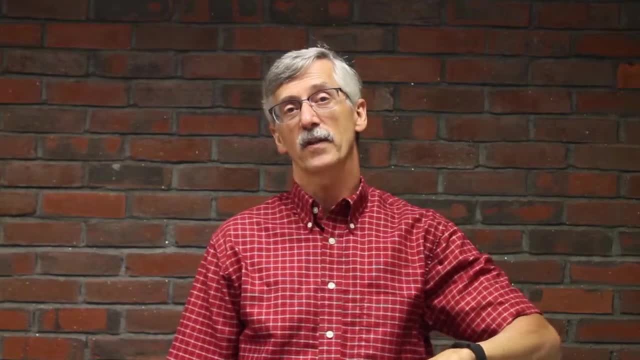 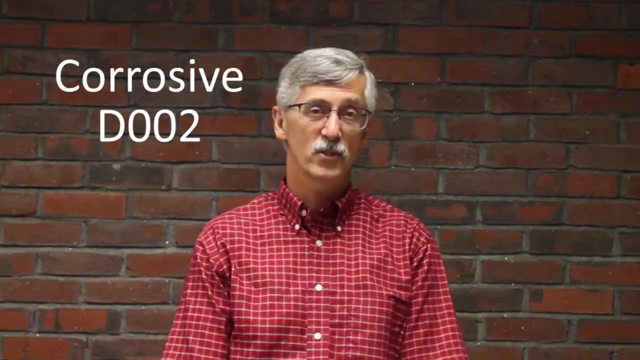 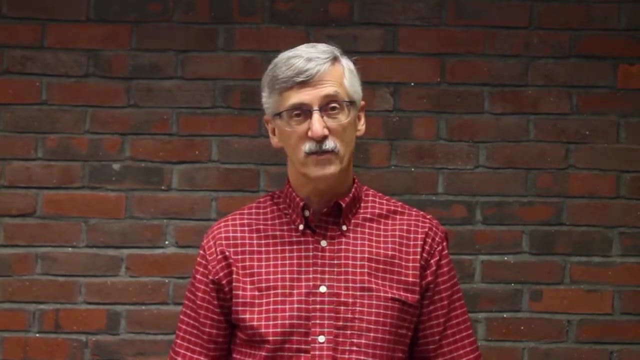 would call caustic or a very low pH, that we would call a strong acid. Things that are corrosive carry a waste code of D002, and we say that if it is beyond a pH range of 2 to 12 and a half. 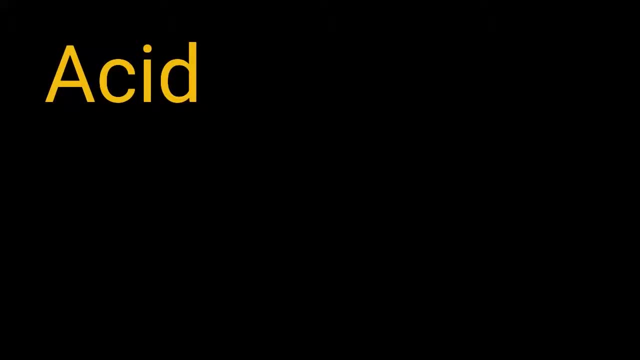 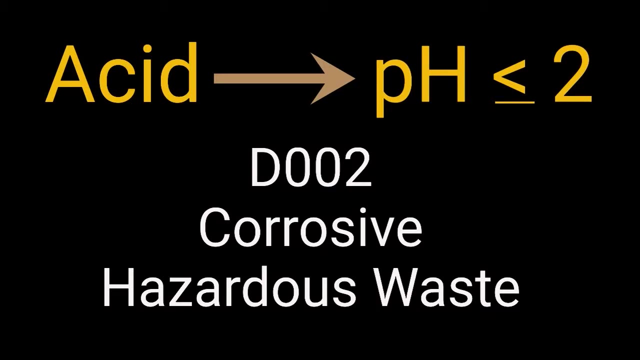 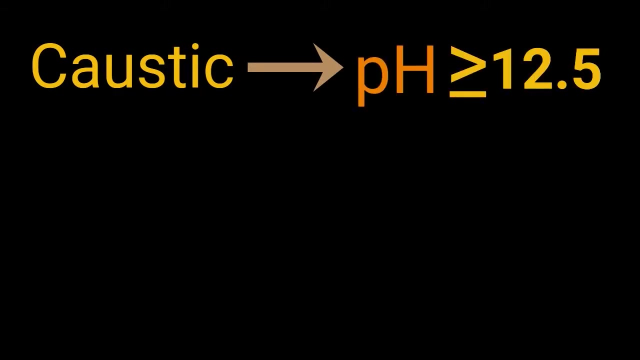 we would consider it to be regulated. So an acid that has a pH of less than or equal to 2 would be a D002 corrosive hazardous waste. If it is a caustic with a pH greater than or equal to 12 and a half, we would say it is a regulated. 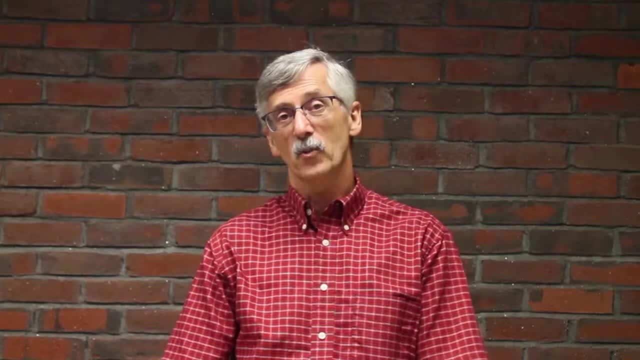 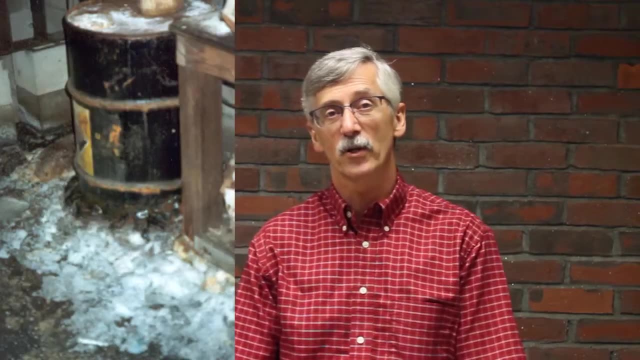 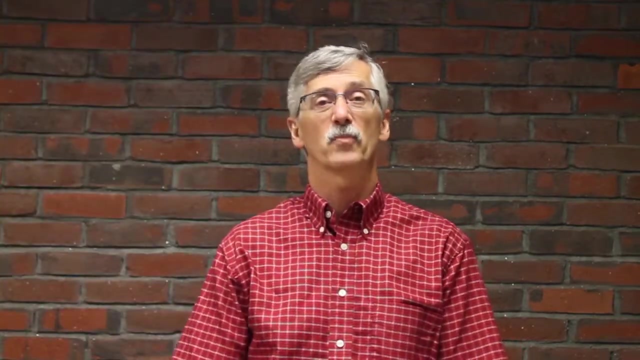 corrosive, hazardous waste. It's also possible in New Hampshire to have something called a corrosive solid. That picture I showed you earlier of the white powder, the container that had rusted on the damp basement floor. that white powder that was filling out, was a. 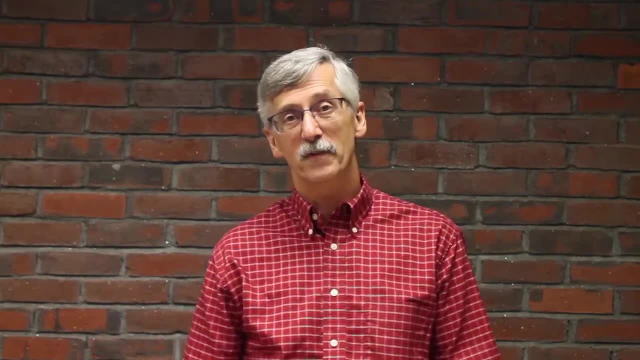 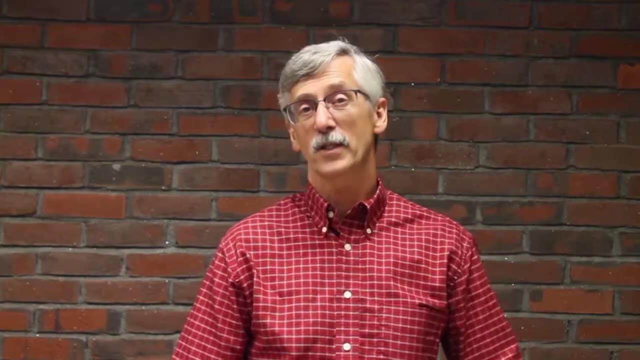 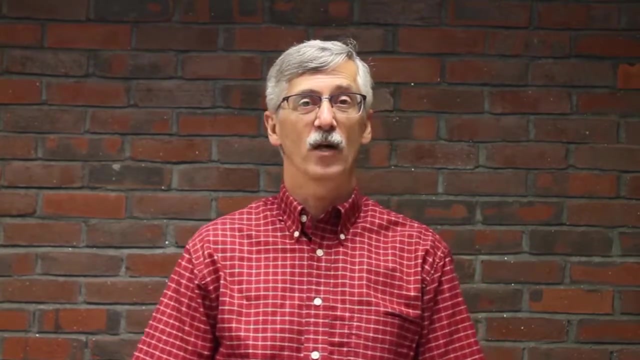 corrosive material. If it had been mixed 50-50 with water and the pH measured, it would have been either higher than or equal to 12 and a half, or less than or equal to 2.. A corrosive, hazardous waste. Here's just some pictures to help you. 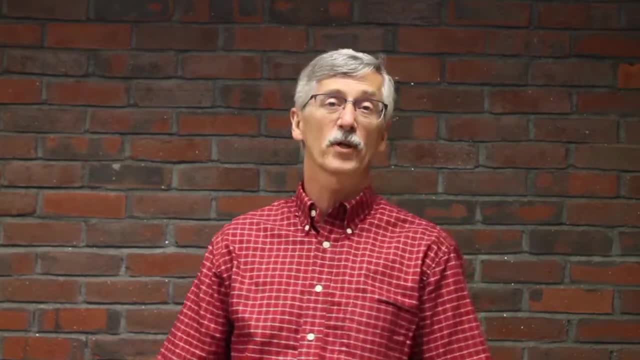 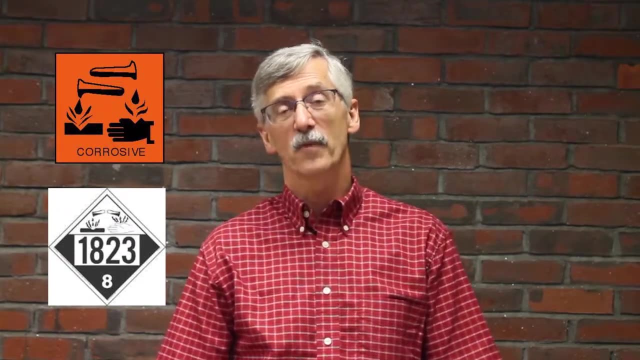 kind of understand, or more clearly understand, what we're talking about. You can easily visualize what a corrosive waste is. On the left some symbols you may look for throughout your facility. On the right is a sample of a pH range for some common 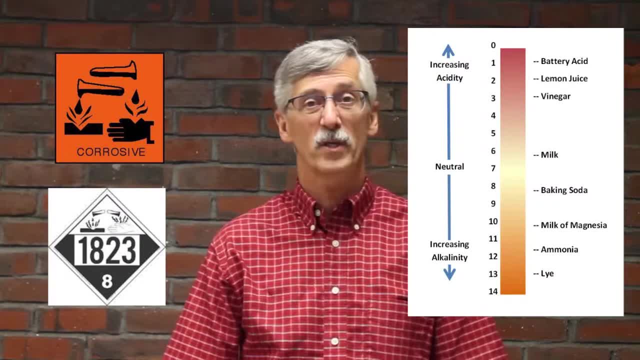 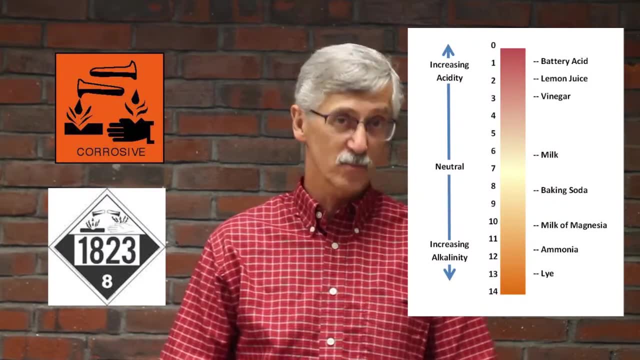 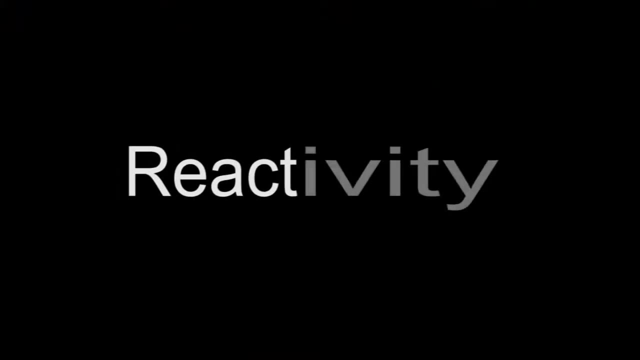 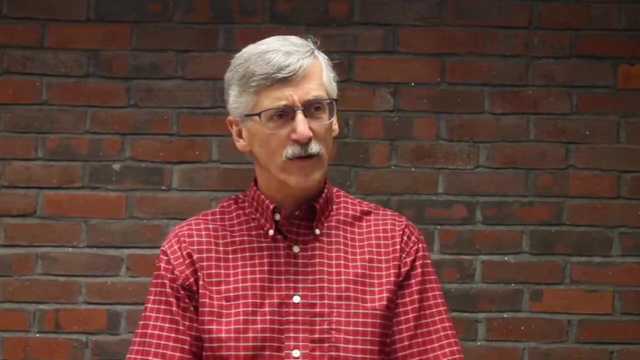 materials you may come across. Lemon juice has a pH of around 2.. A pH of 12 and a half is somewhere between ammonia and lye, So some pretty aggressive chemicals that you are looking at there. Our third characteristic is reactivity. One way to think of reactivity is things. 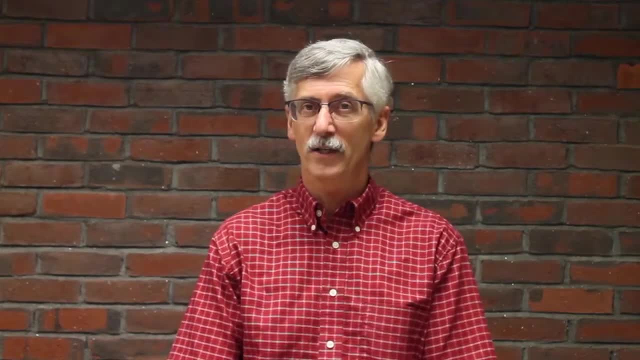 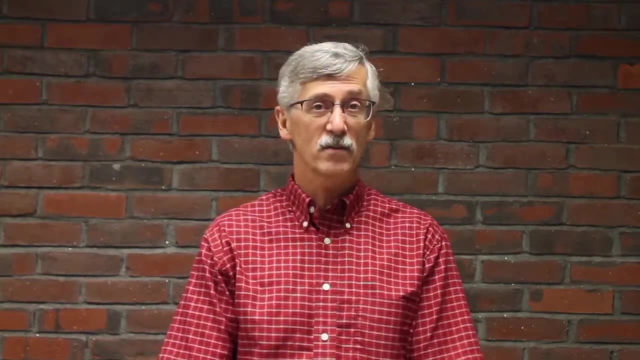 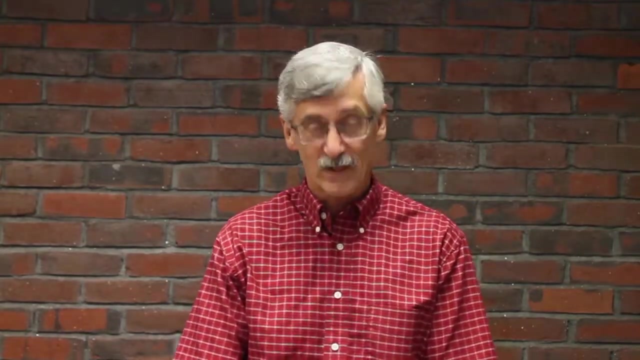 that like to go boom. So if it's something that's inherently unstable- maybe shock-sensitive likely, it's reactive. If it is a waste that reacts badly with water or air, we would say that is reactive as well. Now a lot of 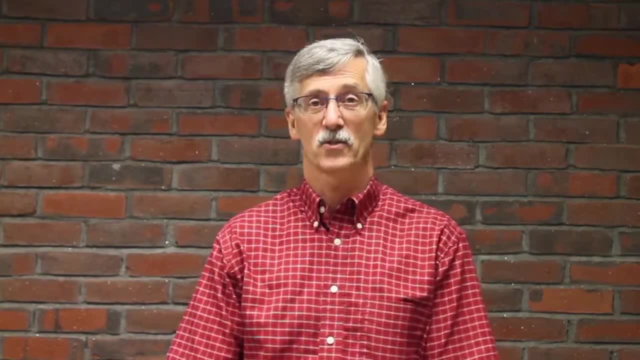 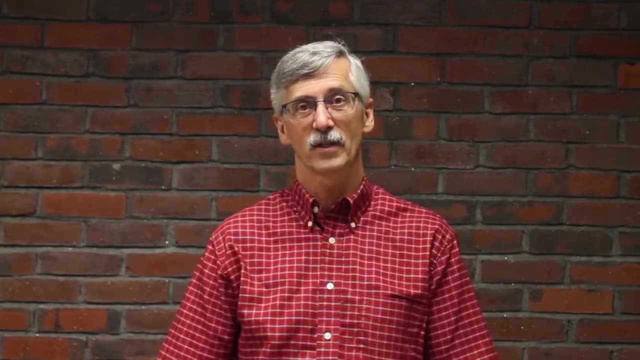 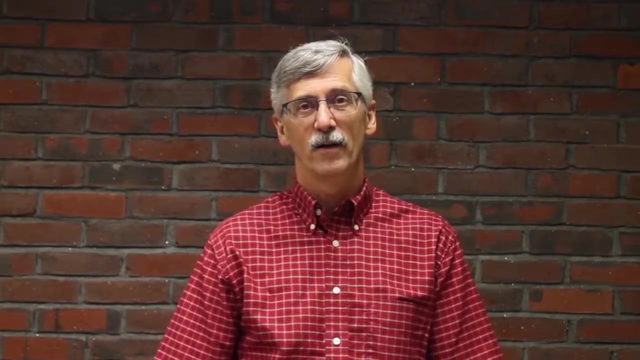 chemicals don't get along with each other. For instance, you wouldn't think to mix ammonia and bleach because we've all been told it creates dangerous chlorine gas and can kill you. But if you have a chemical that's dangerous in contact with water or air, think how difficult it is to avoid those two things. So for that reason we regulate these reactive wastes rather strictly. Another reason a waste could be reactive is because of its high content of cyanides or hydrogen sulfides, Or if USDOT has considered it a forbidden explosive. 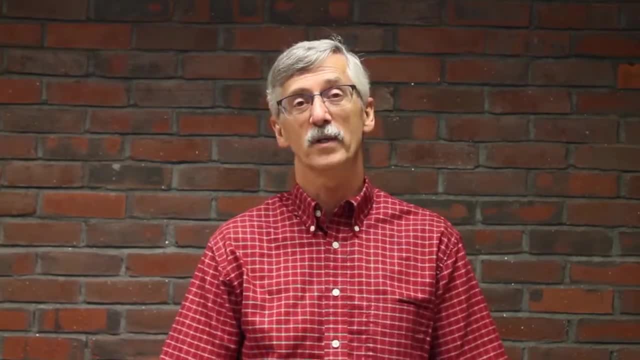 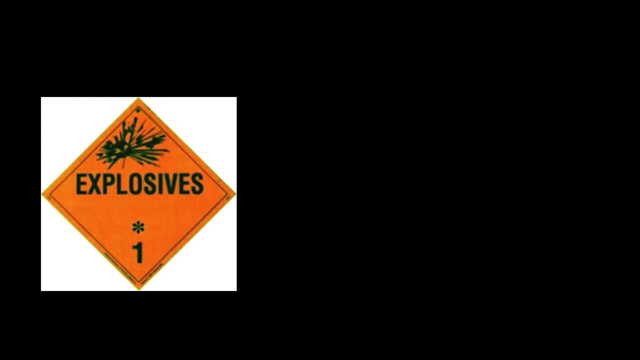 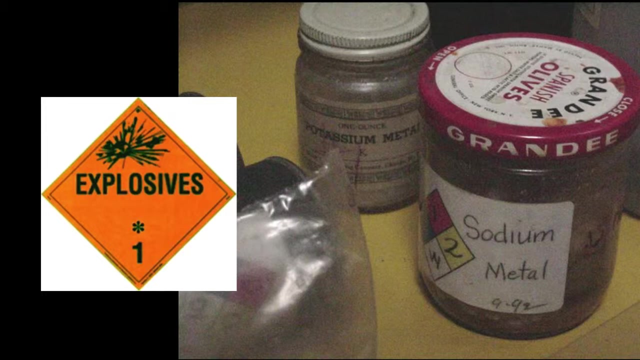 things like dynamite that are wastes we would consider reactive, hazardous wastes. On the left, a symbol you may see to help you identify something as reactive, And on the right, a couple containers of a material that is water reactive. We have two metals, potassium and sodium. 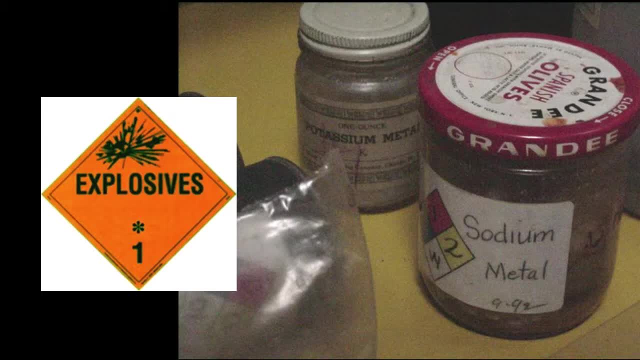 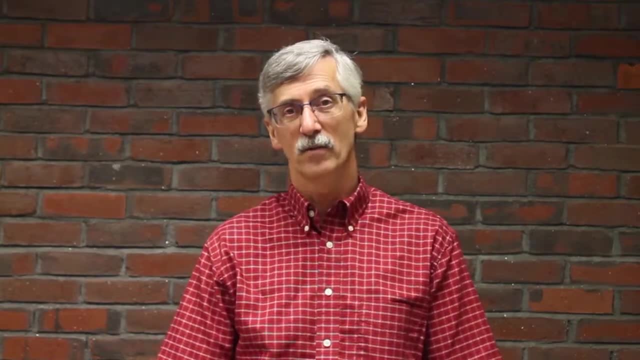 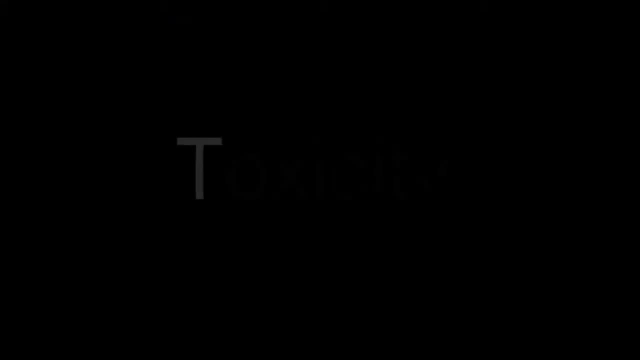 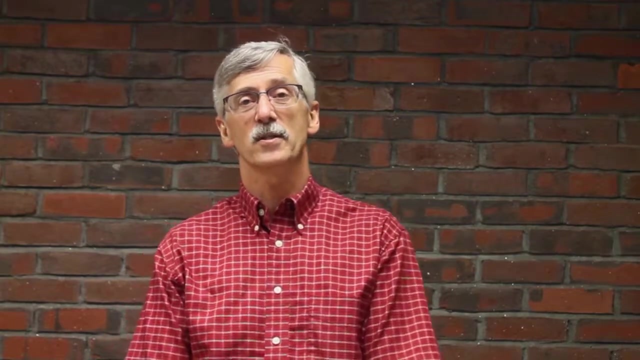 That if they come in contact with water and air, they can burn or even explode. If you come across a container of material that's packed in oil, that may be a good indicator to you that something is water or air reactive. Our last characteristic is toxicity: Things that are dangerous to human. 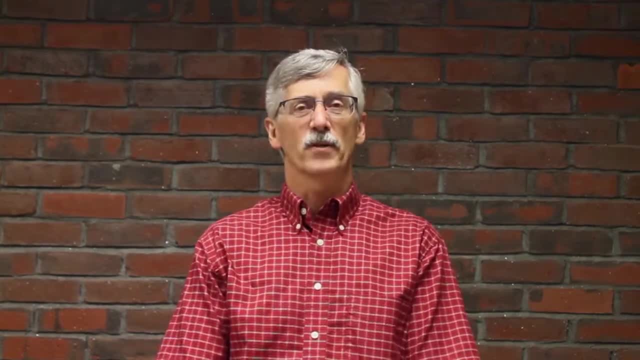 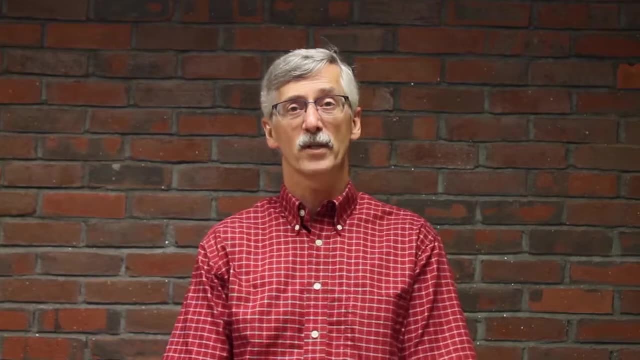 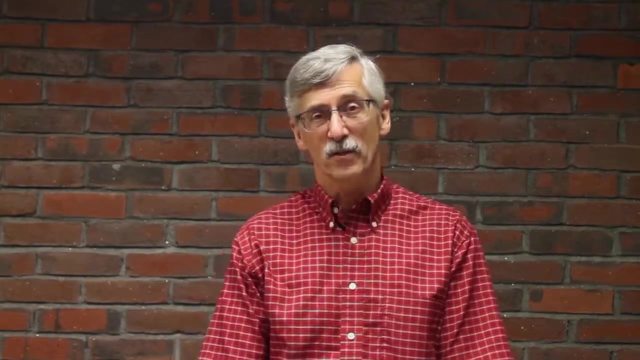 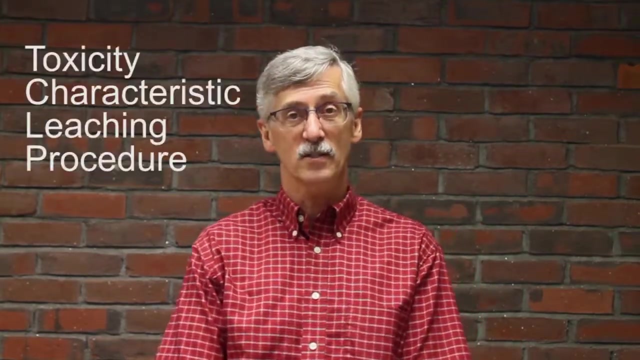 health or the environment. In our rules, there are 39 different metals and chemicals that we are concerned with if they are above a particular regulated concentration. The way that the concentration of these regulated materials is found is using a laboratory test known as the Toxicity Characteristic Leaching Procedure, or 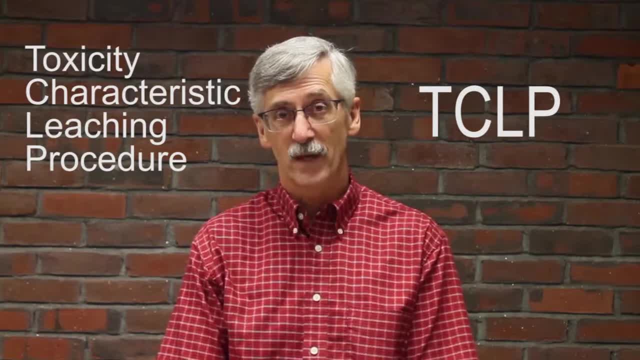 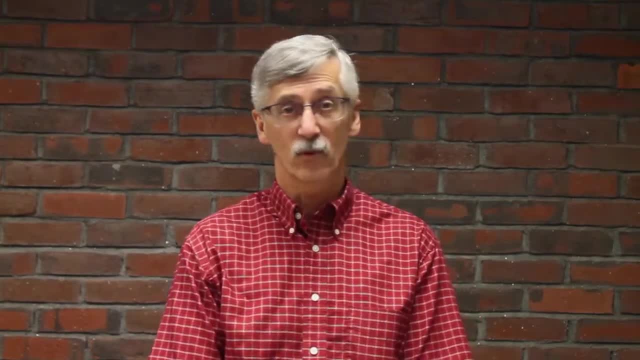 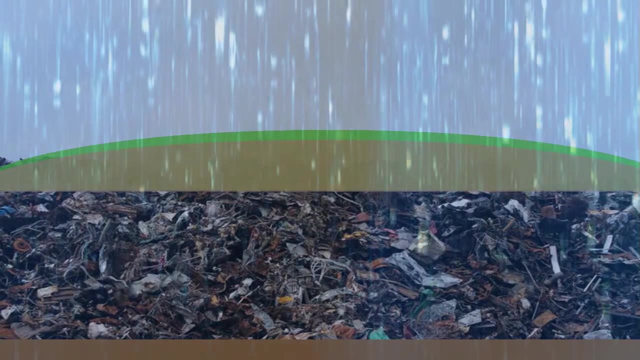 TCLP, also called the T-clip. The way this test is designed is to try and identify what would happen if your waste was placed in a landfill. In New England you get mildly acid rain. lands on the ground, percolates down through the soil. perhaps gets it a little bit more acidic on the way. 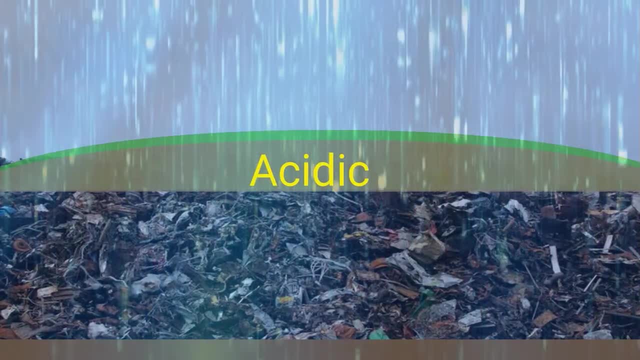 And then when it gets to your waste buried in the ground, it's going to leach or strip out some of the bad stuff that's in that waste. It will continue to carry on until it gets to your waste. But if it gets buried in the ground, it's going to leach or strip out some of the bad stuff that's in that waste. It'll continue to carry on until it's gone. 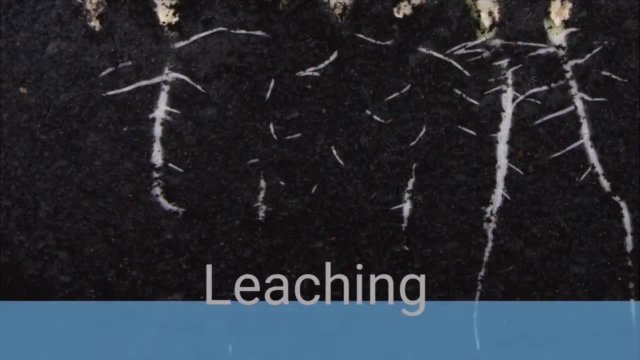 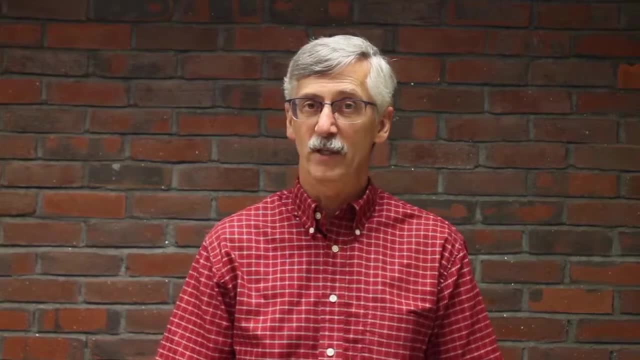 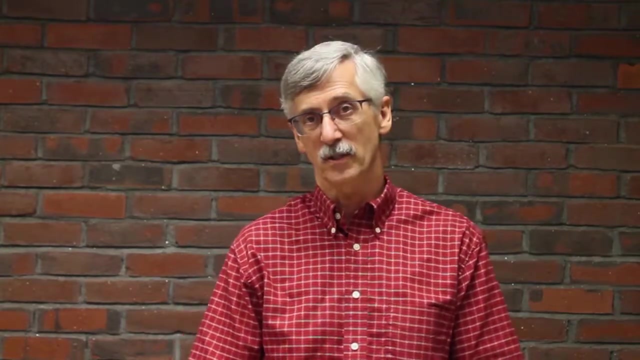 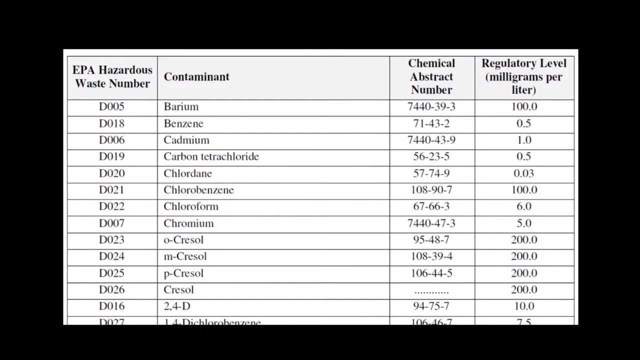 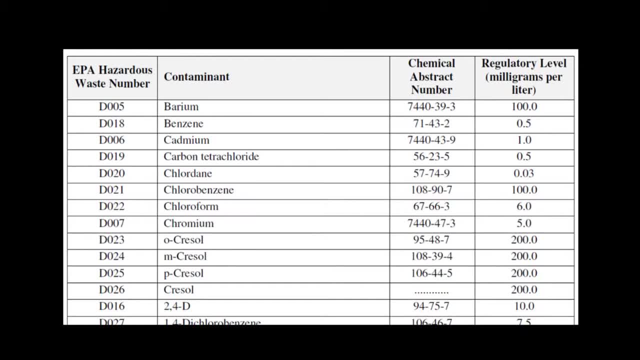 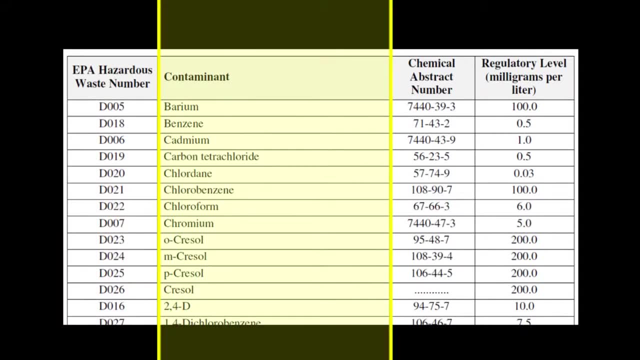 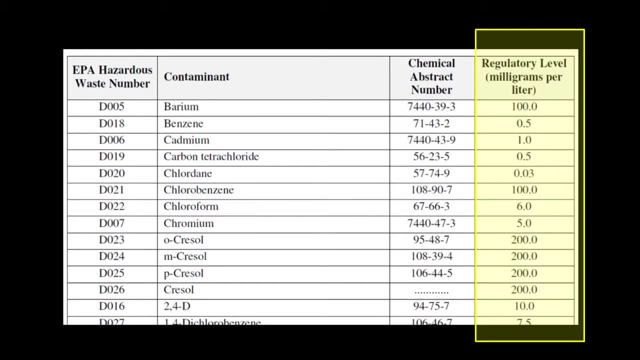 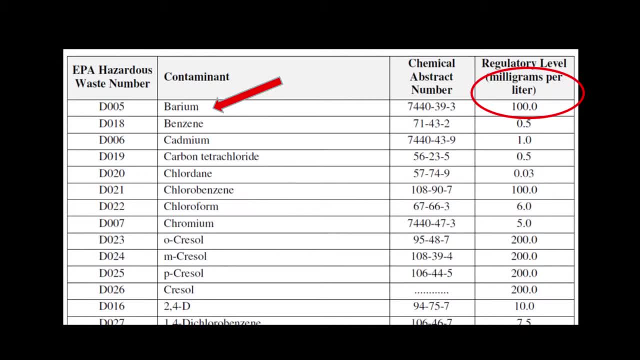